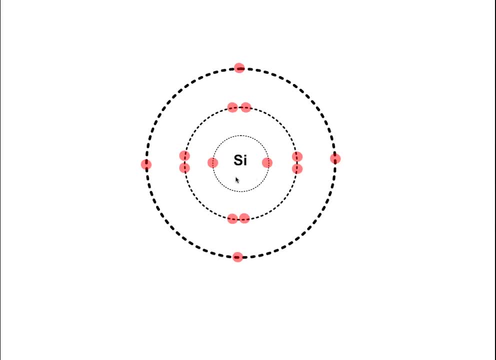 arranged in shells around it. In this case, we've got two in the innermost shell, another eight in the next most shell and then finally four in the valency shell. Now, this valency shell has a tendency to be wanted to be full, And so in this case, silicon could either donate those four. 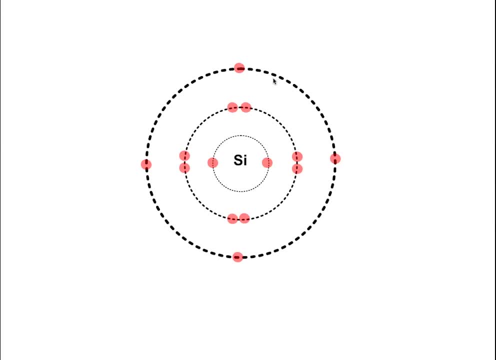 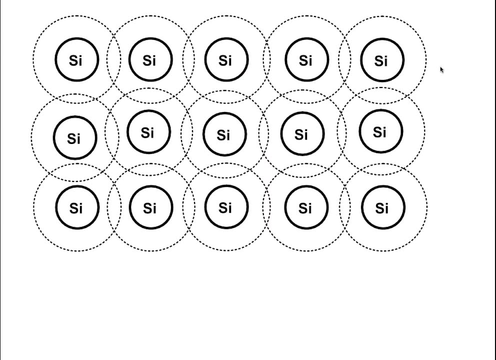 electrons, or it could receive four electrons to become very ionic. But most of you chemists already know that's not what silicon does. So silicon instead forms covalent bonds, And so what happens is is silicon is surrounded by a whole bunch of other silicon atoms. here 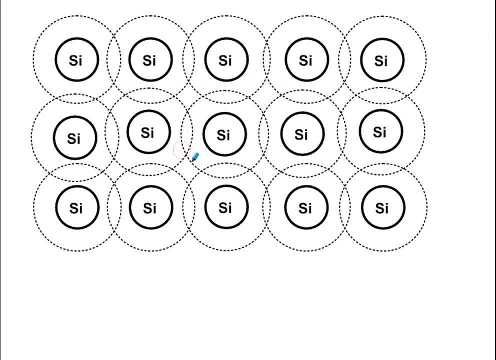 And what happens here, of course, is that here we have the outermost shell And this outermost shell, the valency cell. of course, this silicon over here has four electrons in it, But what happens, of course, is that it, as a result of sharing, 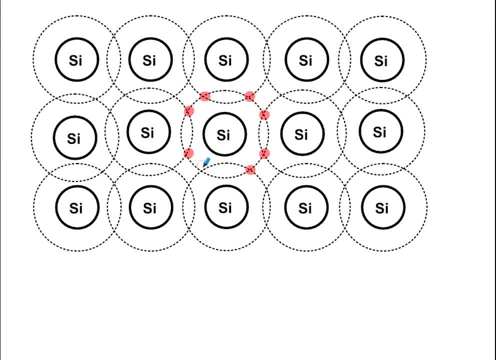 with the neighboring four electrons in the silicons next to it, it creates these four covalent bonds, And so that of course continues throughout. So this outermost valency shell here obviously is now full, but really it's full because of the sharing that's going on And 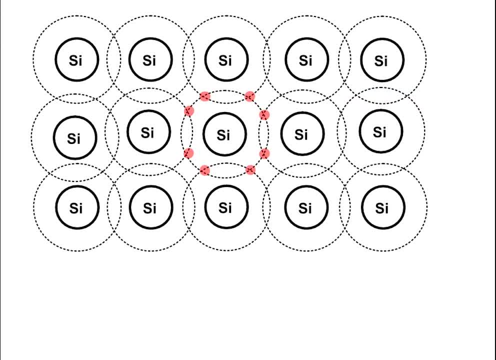 that's called forms, covalent bonds. Now, just before I go on in terms of the band structure, what do you think might happen if somehow I were to remove this one electron? Now, if I remove this one electron and we won't worry about where it goes or what happens to it, 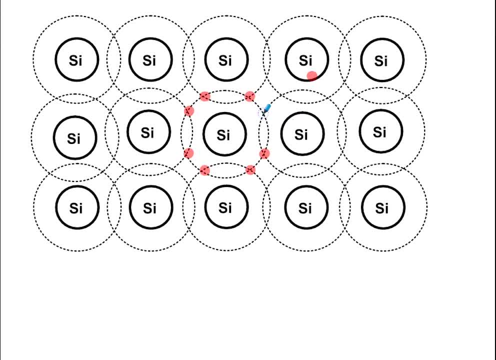 what's happening over here? Well, of course, over in this region, over here, we have now a place where there is a missing electron And, as a result, we would call this maybe a bit as a positive hole. This silicon has lost an electron, but it hasn't lost any protons, So it's now slightly 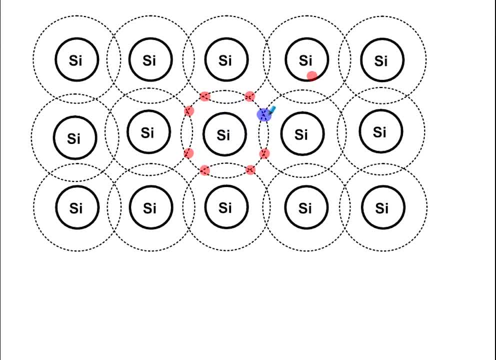 positively charged, But we can call it a hole because it actually is at a slightly higher energy state And this electron could come back And fill it again and then it becomes more stable. So it's a bit like a description of taking some dirt out and therefore leaving a hole behind, And that is really important to understand when 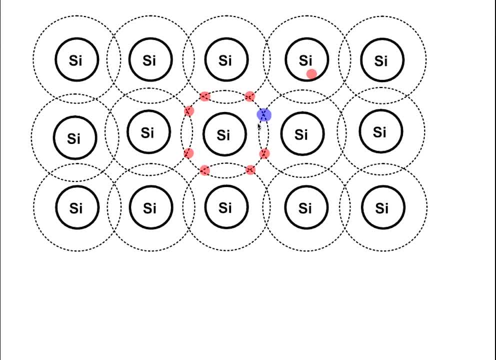 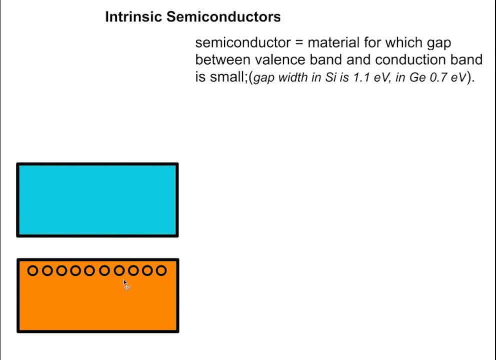 we start talking about how we can explain what happens here under the band structure. So here I have, of course, our band structure And this is silicon And here we have our valency. So here's our band structure And, of course, as I've told you previously, in understanding the 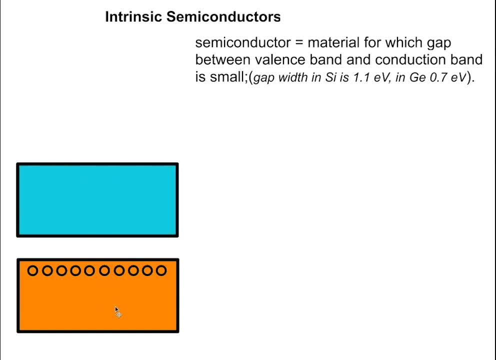 band structure is that we have the conduction band here and the valency band here And there is a small forbidden gap In terms of silicon, which is the one that we're using at the moment. that gap is about 1.1 electron volts. It's a little bit smaller in germanium at 0.7.. 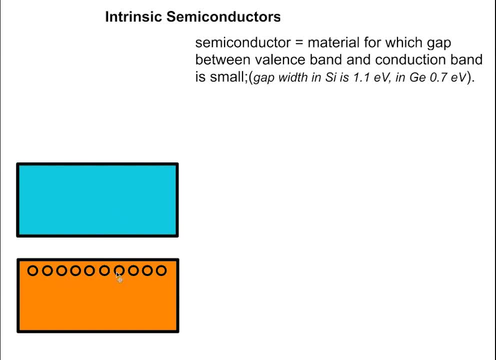 Now, in this case, I have all my electrons bound in their bonds, as they are shaped, bearing, And, of course, at T equals zero, no electrons whatsoever are able to go into the conduction band. That energy, in order for them to move that forbidden gap, has to be contributed by 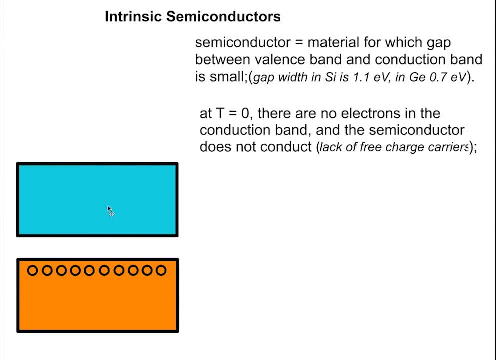 thermal energy, And so, as a result, silicon- at T equals zero, and we own Kelvin degrees, of course- is actually an insulator. It doesn't conduct any electricity. But what happens if I increase its temperature? Well then, some of these, 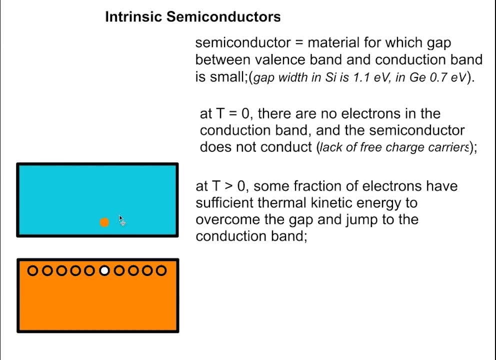 electrons are able to traverse the forbidden gap and move into the conduction band, leaving that hole behind, And if you remember the analogy I gave you just before. And so, as a result, we now have an electron that is free to be used in conduction, If I increase, 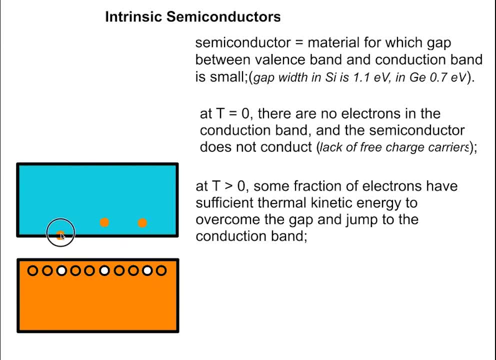 the temperature, more more of these electrons will move into the conduction band. Notice, though, that the number of electrons over here in the conduction band is equivalent to the number of holes that I create In the valency band. It's interesting to note that Faraday actually observed this when he actually 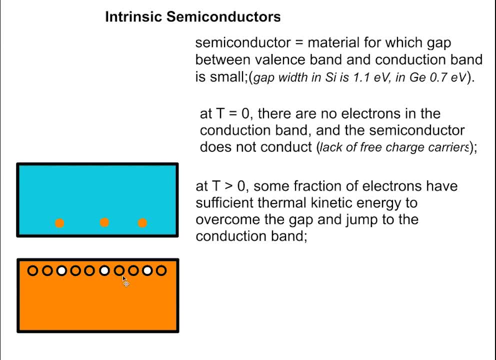 was playing with semiconductors, He noticed quite unexpectedly that increasing the temperature increased the conductivity of a substance, which was sort of against the grain of our understanding of metals, which we know. of course, decreases in conductivity as the temperature increases. Interesting to denote that the increase in temperature has a significant 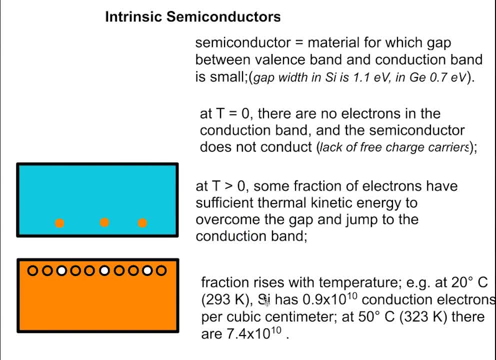 impact on the conduction of a substance, And so we know that the increase in temperature has a significant impact on the conductivity of the material. So, at 20 degrees, or 293 Kelvin, silicon has about 9 billion conduction electrons per cubic centimeter If you increase it to 50 degrees, which is only a small. 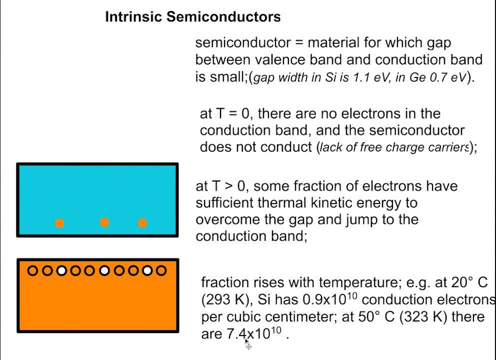 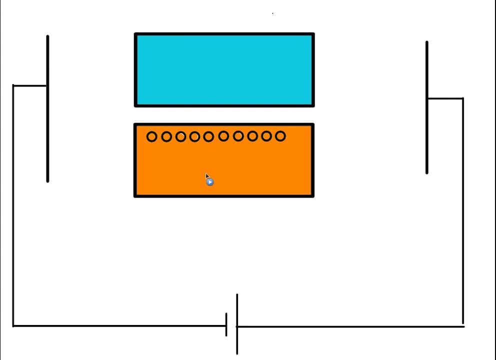 increase. in terms of Kelvin, there's now 74 billion conductive electrons in the conduction band. But let's now have a look closely at these two and ask ourselves the question: what happens if we operate on a conductive electron band? apply a potential difference across the two? well, of course, of a potential difference, you should all. 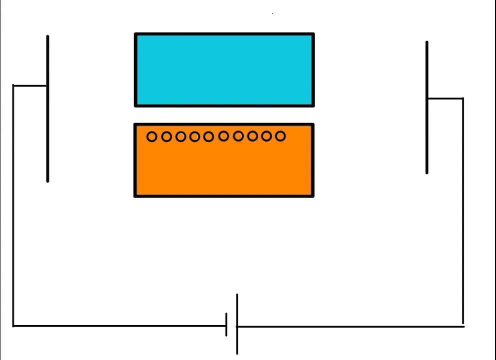 remember that basically, that means this plate over here is got basically positively charged and over this plate here is negatively charged, and so, as a result, you can either argue that we have a potential difference across this, and of course that forms an electric field with electric field lines running in the direction towards the left. so now, if we start heating up the material, 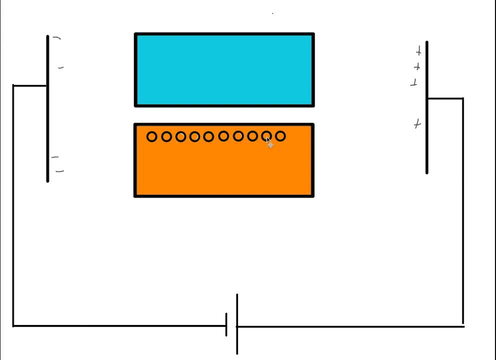 what happens, of course, is is that some of the electrons jump into the conduction band like so, and, of course, as a result, these particular electrons are free to move in this direction, and so what we end up getting is conduction, and rather than talking about electrons, it's useful. 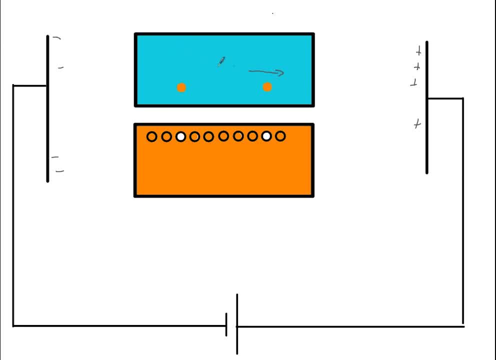 now to talk about the electric field lines running in the direction towards the left. we'll start by talking about the fact that these over here are negative charge carriers. but what happens in the valency band? electrons do not actually move in the valency band and that's. 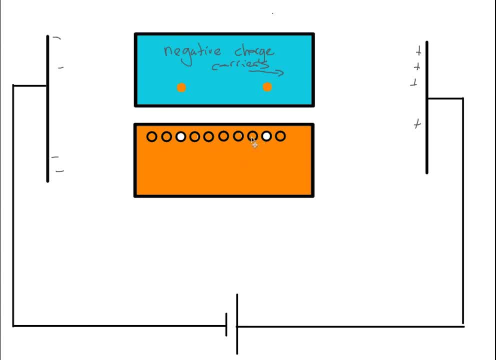 true, but what happens is that these electrons here might move across slowly and surely to the x direction, and in that direction they move in a way that is more or less correct. so the neighboring hole, And if you look very carefully, you'll notice that the white holes,